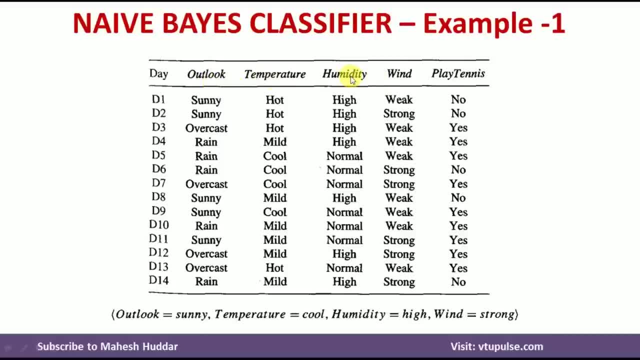 case, namely outlook, temperature, humidity and wind. Platinus is a target variable with the two possible outcomes: One is no and another one is yes. In this case, we have been given a new instance with certain conditions. We need to check whether the new instance can. 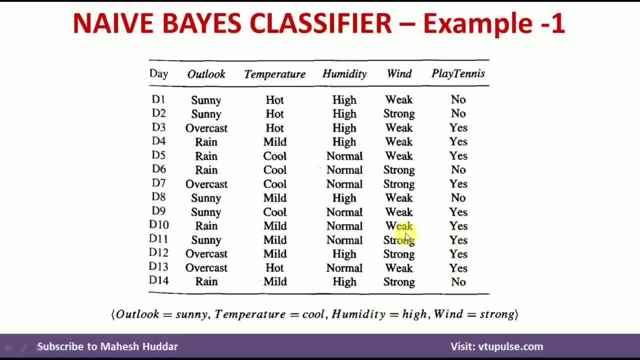 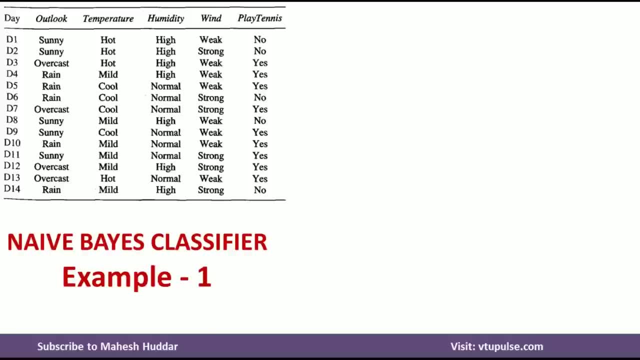 be classified as either yes or no. Now, if you want to classify the new instance into either yes or no or one of the categories, very first thing what we need to do is to calculate the prior probabilities and then the current probabilities. So, the prior probability. 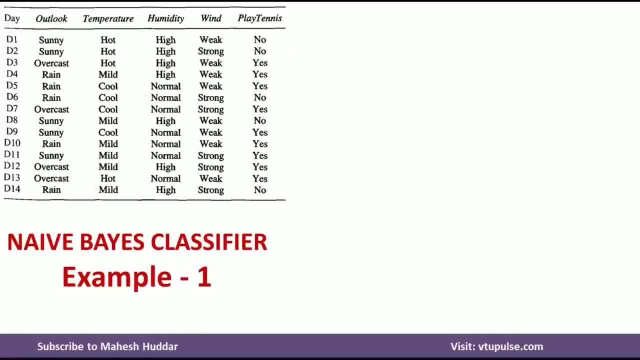 is in this case is the probability of yes and probability of no. So if you count the number of times, yes is appearing. yes is appearing 1,, 2,, 3,, 4,, 5,, 6,, 7,, 8 and 9. number of time: 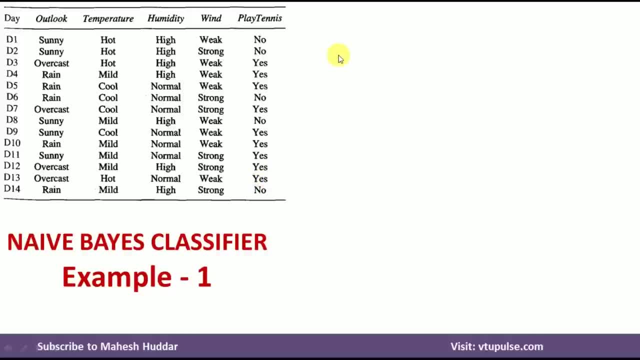 So the probability of yes is 9 by 14 and the probability of no is 5 by 14.. So this is the prior probability. Probability of platinus is equivalent to yes, which is equivalent to 9 by 14.. Probability that platinus is equivalent to no, which is equivalent to 5 by 14.. Once, 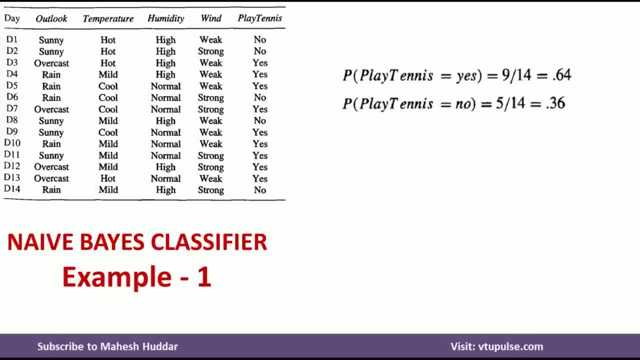 you calculate the prior probabilities. next we need to calculate the current probabilities. that is also called as conditional probabilities. Here we have four attributes: outlook, temperature, humidity and wind. We need to calculate the conditional probabilities of all these attributes. Here I have written the attribute name and. 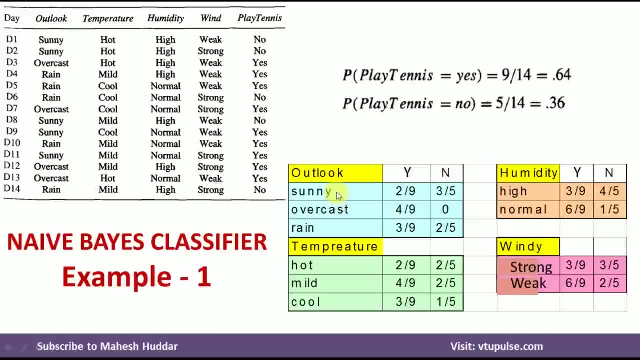 the possible outcomes of this attribute is written here, and these are the possible values of this attribute. Now, we know that there were five yes examples are there. We know that there are nine yes examples are there and five no examples are there. Out of this, nine and five yes and no examples, we need to count how many number of times. 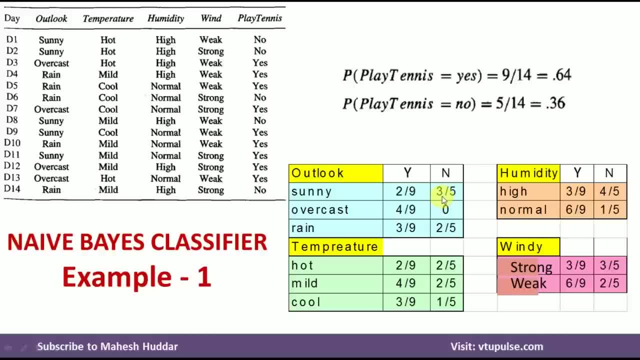 sunny is appearing in yes and no respectively. Similarly, how many times overcast is appearing in yes and no respectively, and rain is appearing in yes and no respectively, So that we can calculate the conditional probabilities. So we can calculate the conditional probabilities. 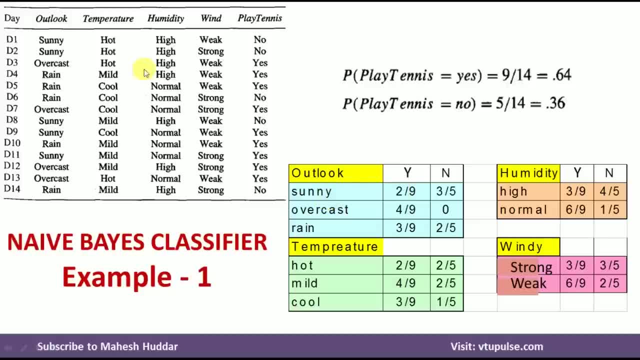 If we count sunny, In the first case sunny is appearing in no examples. second one is no, third one is no, fourth one is Yes and fifth one is yes here. So there are two Yes examples are there and the three no examples are there. That is, 2 by nine is the probability. 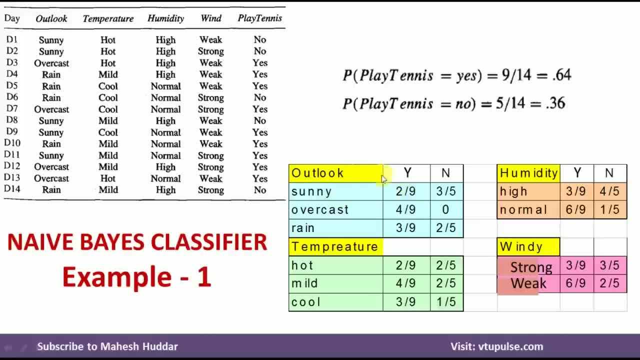 that outlook is equivalent to sunny given yes And three by specialhhhh. yes, here blocks ET. if continue, then probability is given inınız, Then probability of sun is given inkan, usually when sun signifies yet only details. So once you plug those two moments, 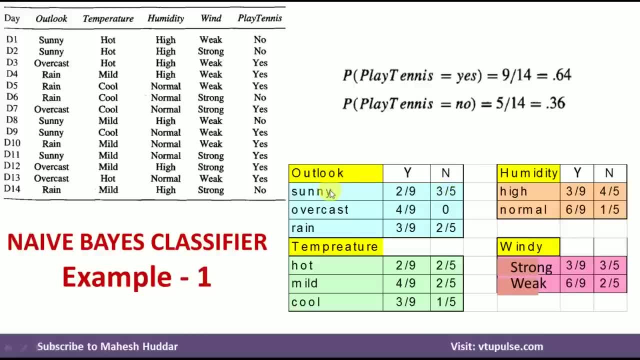 0 by 5 is the probability that outlook is equivalent to sunny, given no. Similarly, we need to calculate it for overcast. Overcast is appearing in S, Second one is in S, Third overcast is appearing in S and fourth one is also in S. So the probability that outlook is equivalent to overcast, given S, is equivalent to 4 by 9.. 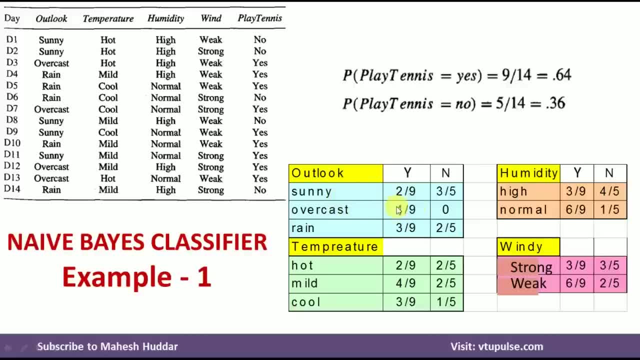 So the probability that outlook is equivalent to overcast. given no is equivalent to 0. by 5, that is equivalent to 0.. Similarly, we need to calculate the conditional probabilities of all the attributes and the possible values of those particular attributes. So this table shows how can we calculate the conditional probabilities. You can pause the video for a minute and try to calculate the conditional probabilities. If you find any difficulty, we can put those difficulties in the comment box. 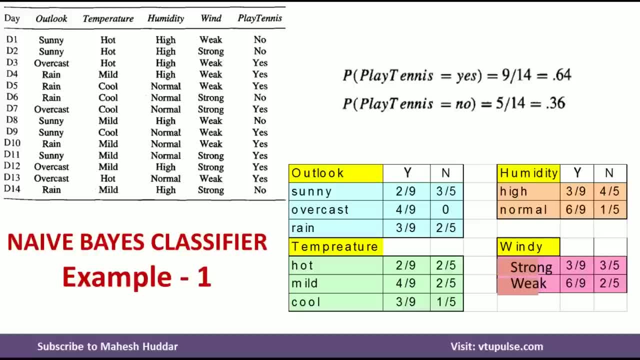 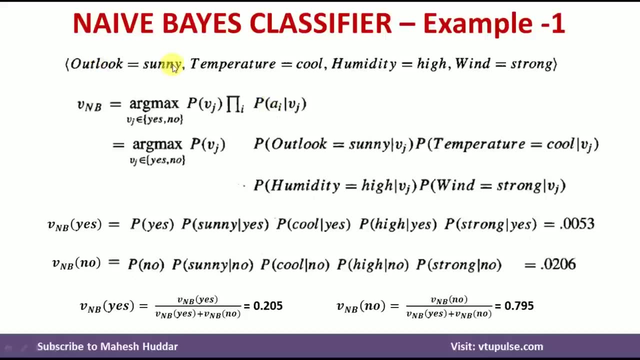 So that we can address those things at the later part. Now, once you calculate the prior probability and the conditional probabilities, the next task is to classify the new instance into either yes or no class here. So the new instance is: outlook is equivalent to sunny, temperature is equivalent to cool, humidity is equivalent to high and wind is equivalent to strong. So these are the conditions given to us. So, given these conditions, whether this new instance belongs to yes or no, we need to find it out. 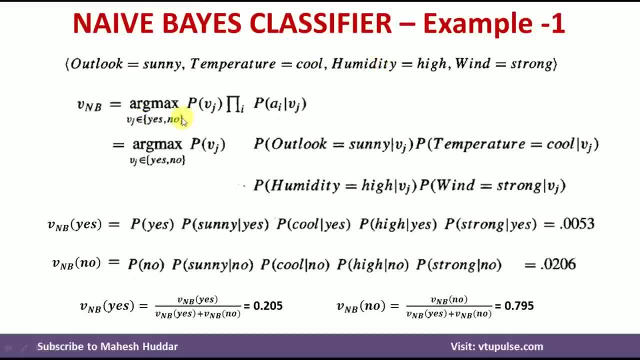 So this is the nearby classifier equation. VNB is always equivalent to argmax of VJ belongs to yes- no. Here, yes and no are the two target values. we have Probability of VJ multiplied by product of probability of AI, given VJ, where AI is the set of attributes and VJ is the possible outcome. in this case, 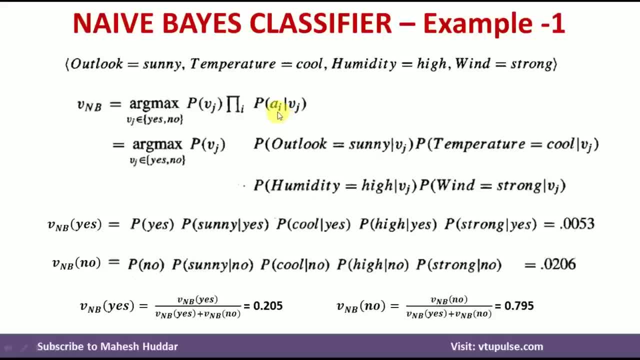 So first we will replace AI with the given conditions. The AI is given like: outlook is equivalent to sunny, temperature is equivalent to cool, humidity is equivalent to high and wind is equivalent to strong. So the same thing. I have written it over here. 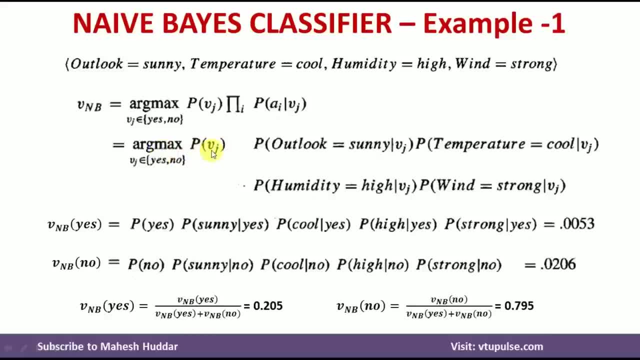 Next, what we need to do is we need to replace VJ by yes first time and no second time, And then we need to calculate the probability. Depending on that probability, we can decide whether the particular person will play the tennis or will not play the tennis. given these conditions, 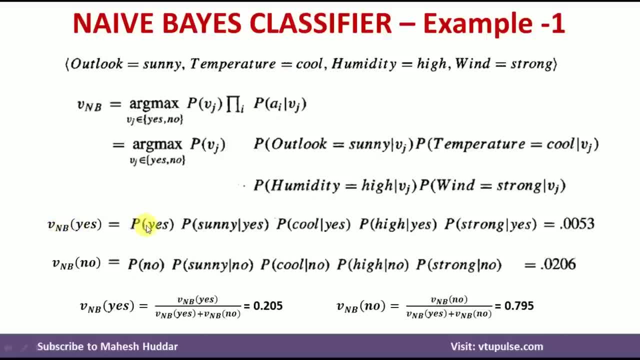 So VNB of yes is always equivalent to argmax of VJ. Now let us try the probability of Panel data. So we need to put the values we have calculated in the previous slide. that is, probability of VJ of sunny. given Yes distributable probability, VJ is equivalent to probability of yes. that is, VJ is replaced by Yes here and this VJ should be replaced by Yes, and so on. 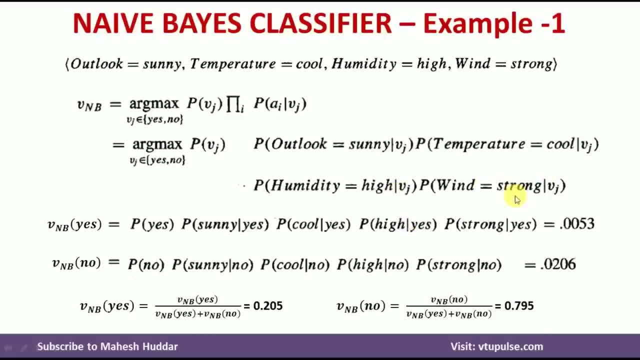 So probability of Sunny, given VJ, that is yes. probability of Cool, given Yes. probability of High, given yes. probability of Strong, given Yes. So we need to put the values, what we have calculated in the previous slide, that is, sistema, the activities, silos, the image armor. 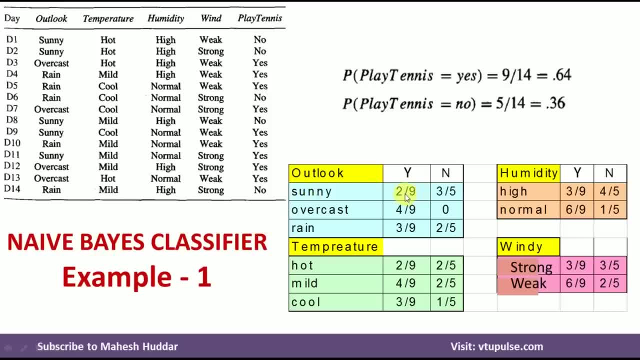 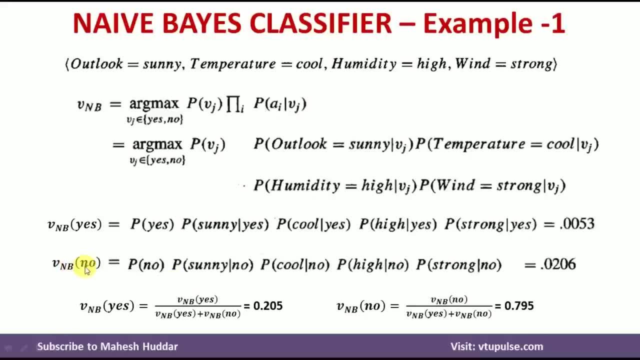 given S is equal to 2 by 9.. Similarly, we need to put all the values here, We will get the answer as 0.0053.. With the same note, VNB of no- we need to calculate that is, VJ is equal to no in this. 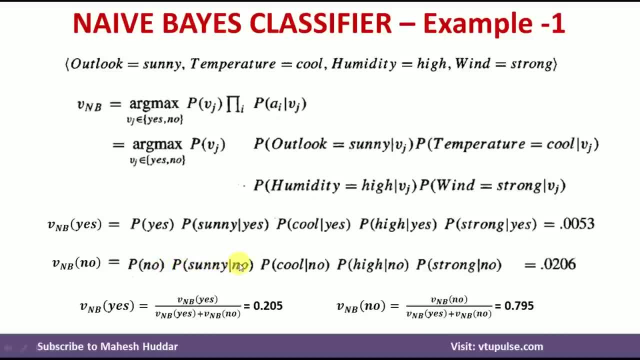 case: Probability of no probability of sunny, given no. probability of cool, given no. probability of high given. no probability of strong, given no. If you put all the values in this equation, we will get 0.0206 as the probability. If you compare these two probabilities, the probability of no. 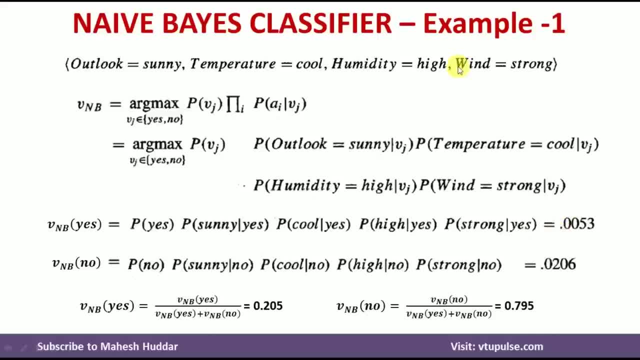 is more than the probability of yes, It means that the new instance is classified as no. The meaning is the person is not going to play the tennis. There is one more thing we need to do, That is, we need to normalize these probabilities, because these are the equivalent probabilities, because 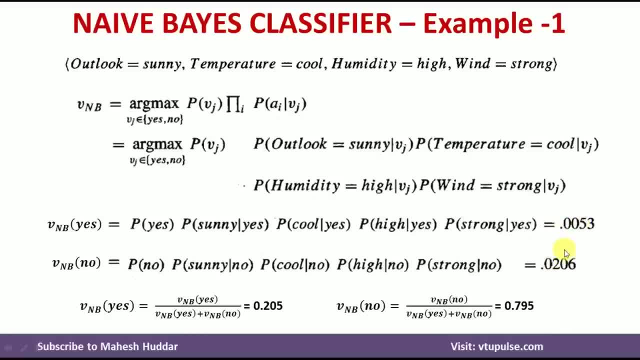 we have removed the denominator term, So if you want to consider that we need to normalize it, The normalized values can be calculated something like this: VNB of S is always equivalent to VNB of S divided by VNB of S plus VNB of no. If you put the values here: